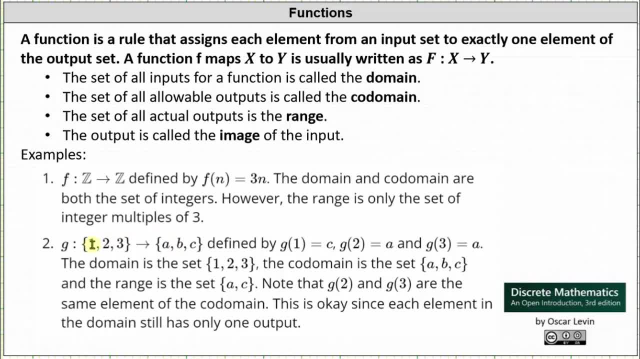 Meaning: the first element of one does not necessarily have an output of a- the first element- in the codomain. The second element of two in the domain does not necessarily have an output of b in the codomain, and so on. We actually have to define the inputs. 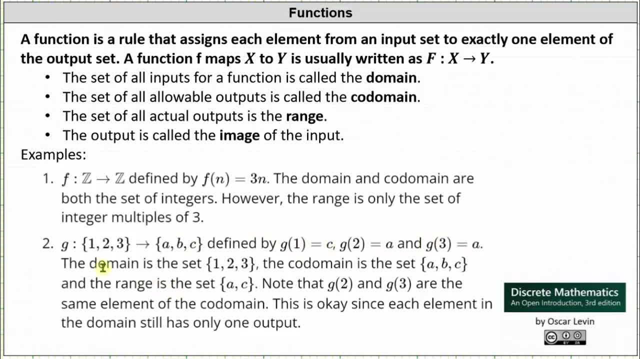 and outputs, as shown here. So in this case, the domain is the set containing the elements of 1,, 2, and 3.. The codomain is a set containing the elements of a, b and c. the range is the set containing only the elements of a and c, because those are the only actual. 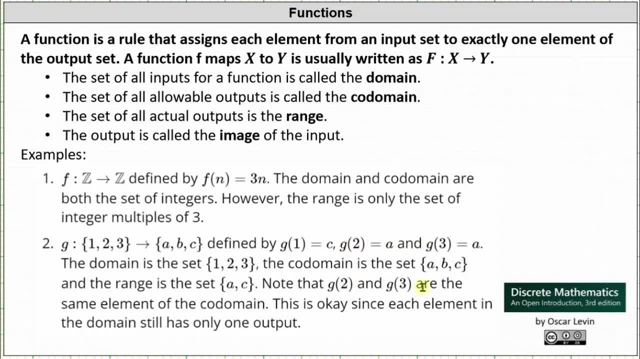 outputs And also notice that g of 2 and g of 3 are the same element of the codomain because both outputs are a. This is okay, since each element in the domain still has only one output. Again, the input of 2 has exactly one output, which is a, and the input of 3 also has exactly one. 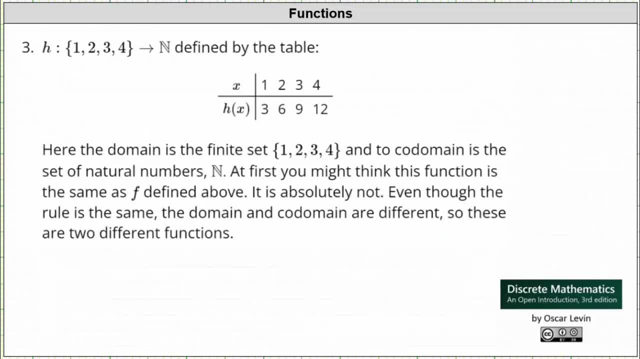 output, which just happens to also be a. And let's look at one more example of a function. Here we have the function h that maps the set containing the elements of 1,, 2,, 3, and 4 to the set of natural numbers defined by the table, where we have the inputs in the first row. 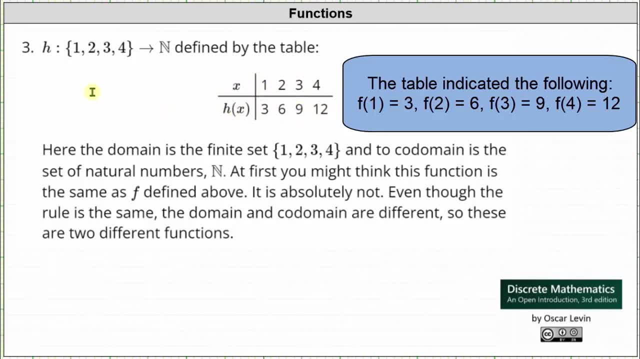 and we have the outputs in the second row. Here the domain is the finite set containing the elements of 1,, 2,, 3, and 4, and the codomain indicated by n is the set of natural numbers. At first we might think this function is the same as the first function f we defined in number 1,. 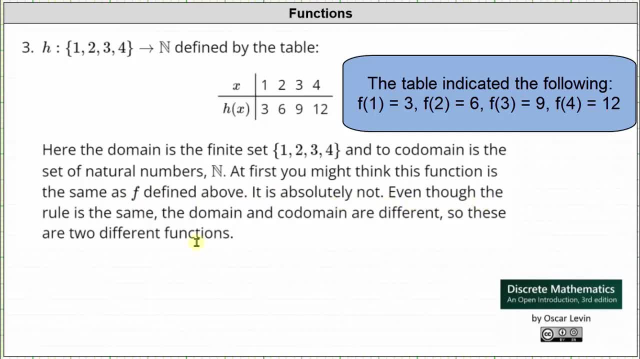 but this is not true, Even though the function rule is the same, because- notice how to determine the outputs. we multiply the inputs by 3, the domain and codomain are different, so these are different functions. If we take a quick look back at number 1,. 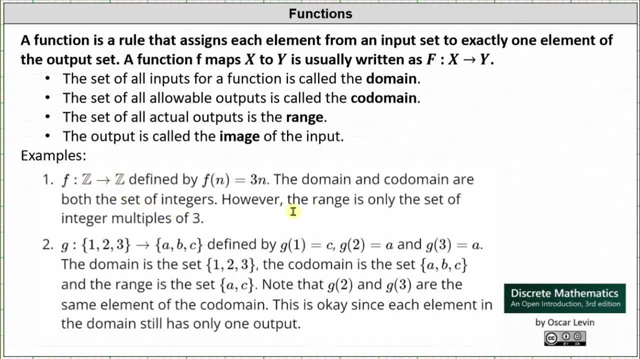 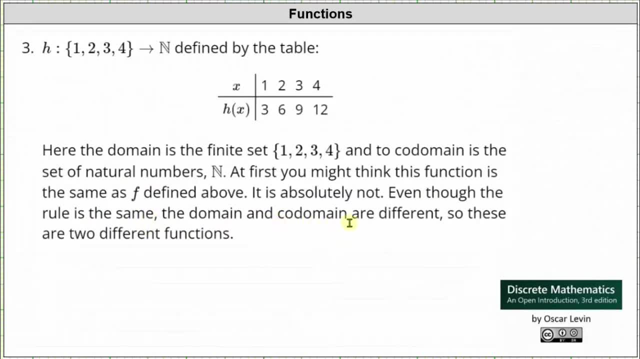 the domain and codomain were the set of integers and the range was the infinite set of integers. So the domain, codomain as well as the range are different, And now let's look at some examples of rules or relations that are not functions.